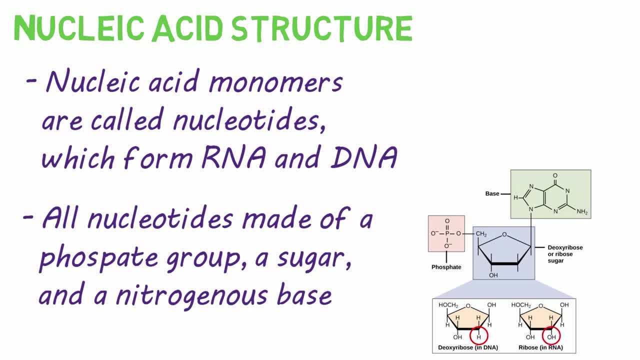 In DNA, the sugar is also a ribose, but with an extra form of ribose on the outside, one less oxygen. Hence RNA is ribonucleic acid and DNA is deoxyribonucleic acid because the ribose has been deoxygenated. 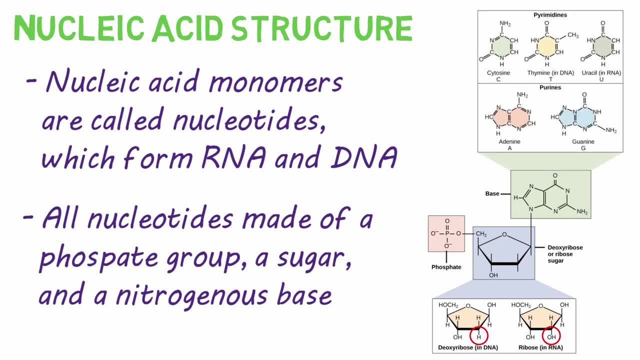 Finally, we have the nitrogenous base, and if you've studied DNA at all, you probably remember these. The nitrogenous bases in DNA are guanine, adenine, cytosine and thiamine. RNA also has guanine, adenine and cytosine, but instead of thiamine, RNA contains uracil. 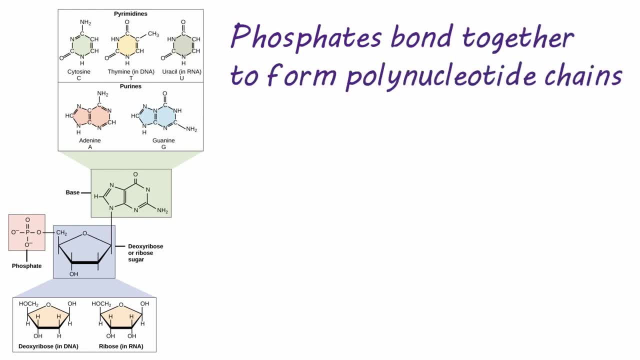 The phosphate of nucleic acids bond together to form long polynucleotide chains like RNA and DNA. The nitrogenous bases can form weaker hydrogen bonds, as they do between two strands of DNA. This bonding gives DNA its helical structure and allows it to perform. 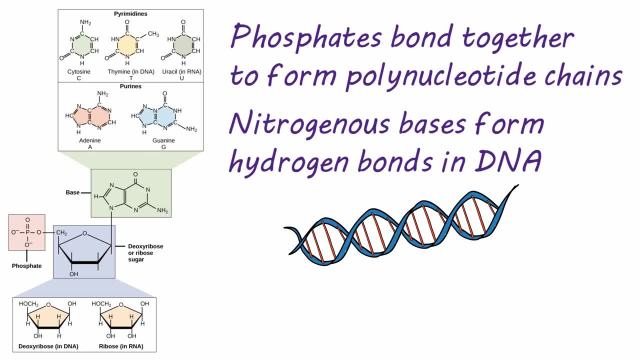 many important functions. Nucleic acids are an underrated molecule, in my opinion. Carbohydrates, proteins and fats seem to get all the attention, but nucleic acids store all the genetic information for your cells. Without them, your body wouldn't build the 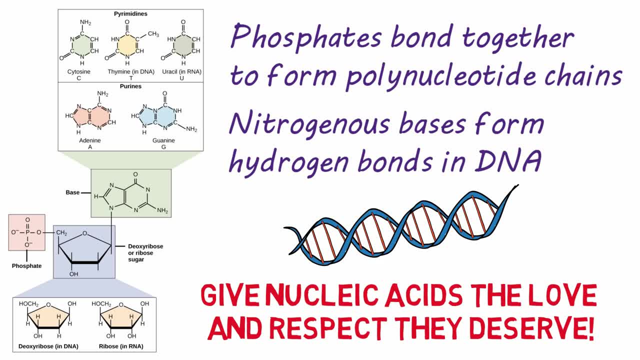 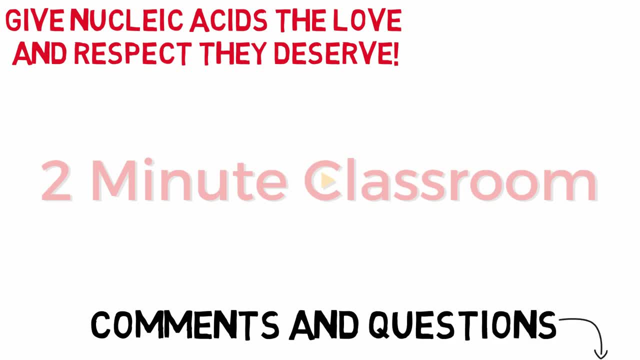 necessary machinery to carry out all cellular functions. I hope this video answered any questions you had. If you still have some, I love to reply to my comments, so send additional questions there. You should also check out my video on DNA vs RNA, which goes into more detail, And don't forget to smash that like button. 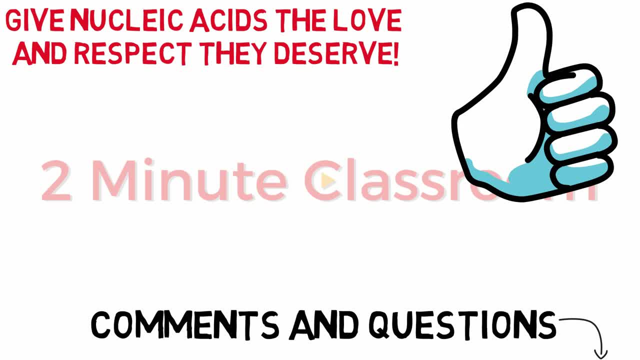 and subscribe for more quality content. I'll catch you next time. See you next time. 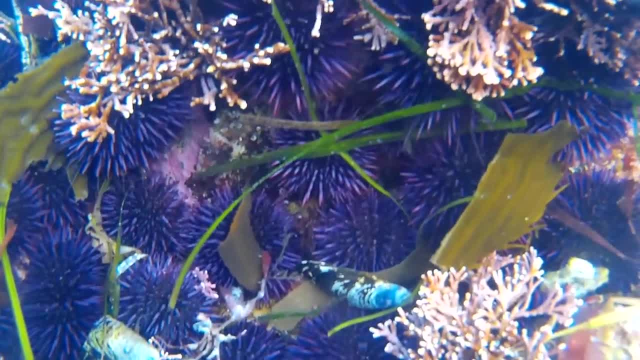 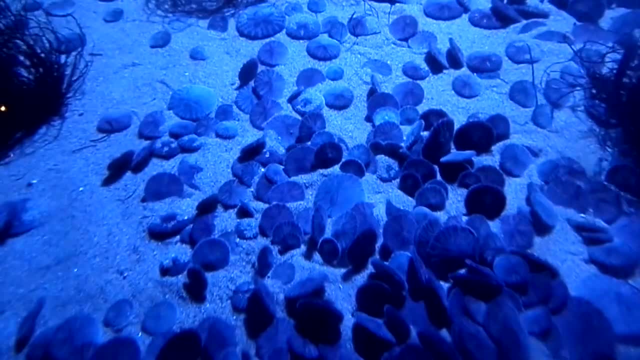 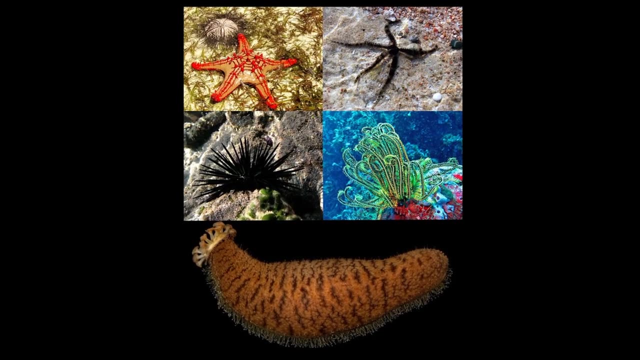 Echinoderms are a group of marine invertebrates that includes organisms like sea stars, brittle stars, sea urchins, sand dollars, sea cucumbers, crinoids and sea daisies. Together they make up the phylum Echinodermida. There are about 7,000 living species. Echinoderms live in every ocean, from warm tropical waters to polar seas, from shallow waters to some of the deepest depths of the ocean. As adults, they usually have a five-point, radially symmetrical body plan, with their circulatory, nervous and skeletal systems radiating in five directions from a central axis,